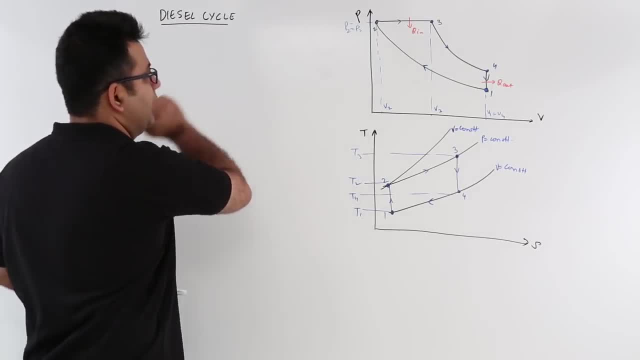 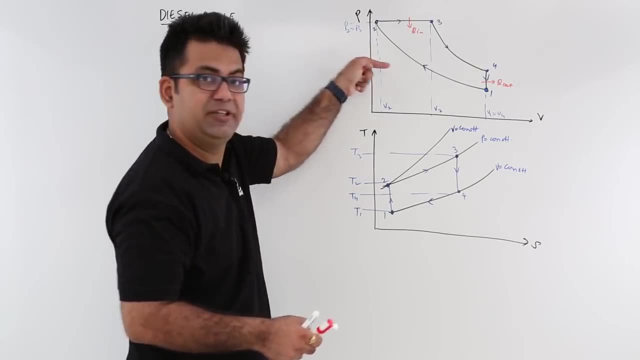 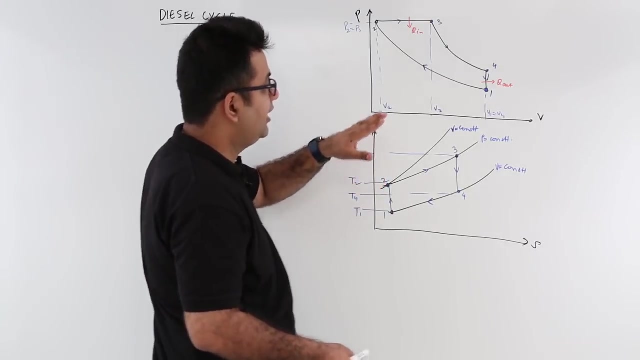 Now let's talk about the diesel cycle. Now the difference between auto and diesel cycle is that in auto cycle you had a constant volume heat addition. You remember that. But in diesel cycle you have a constant pressure heat addition, But the heat rejection is always at constant volume. 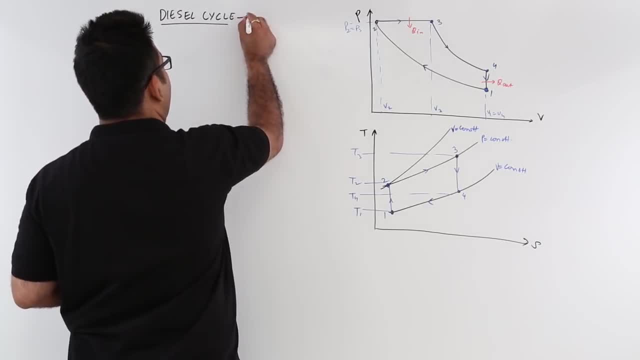 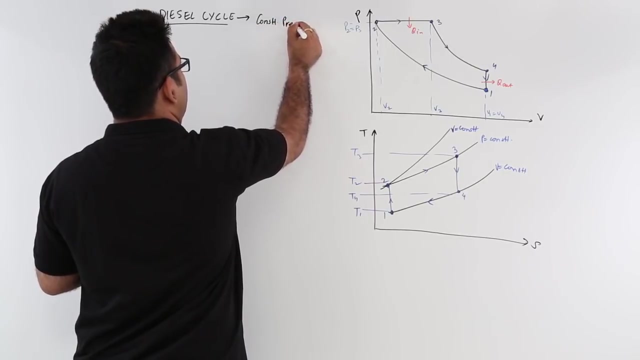 So the diesel cycle? as we all know, this is a working cycle for all the diesel engines or compression ignition engines, So the diesel cycle is also alternatively known as a constant pressure heat addition cycle. Heat addition cycle- Alright, So this is what you have. 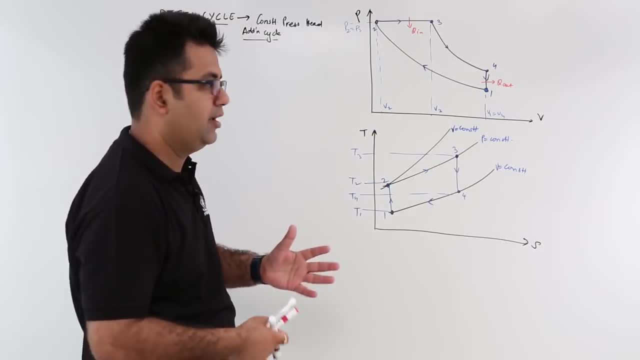 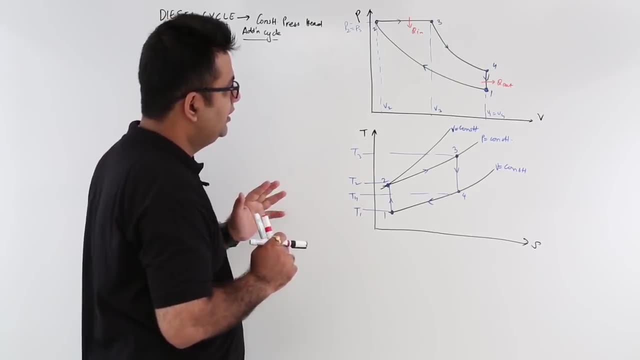 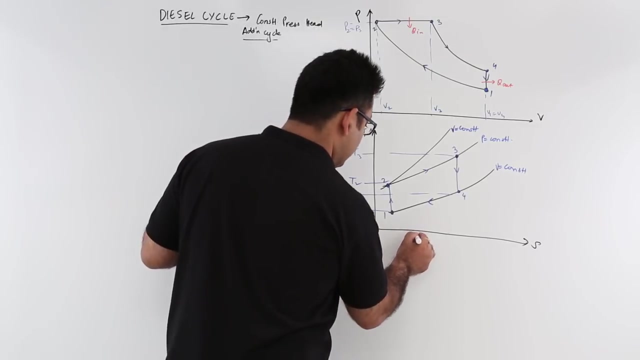 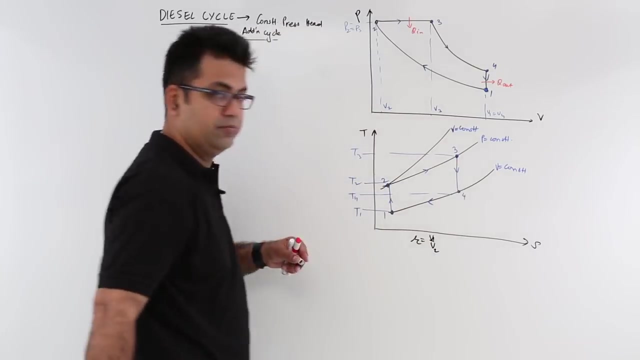 Now let's get to the analysis of it and try and find out some expression for the efficiency. Before we do that, there are three ratios. we need to understand The first ratio but of course the compression ratio. so that is R, which is equal to V1 by V2.. V1 by V2.. That is the volume before compression by volume. 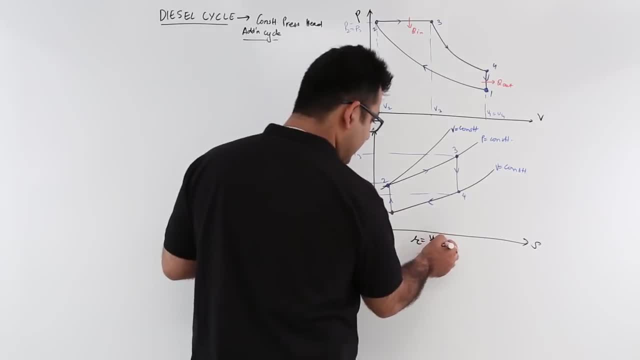 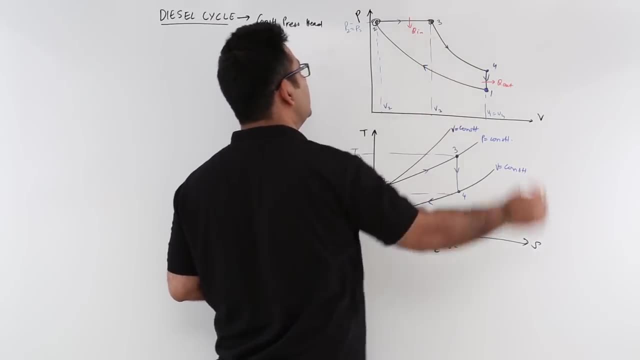 of after compression. Now, the second is the fuel cutoff ratio. So the fuel starts to get supplied at 2 and it finishes at 2.. So the fuel starts to get supplied at 2 and it finishes at 2.. So the fuel starts to get supplied at 2.. 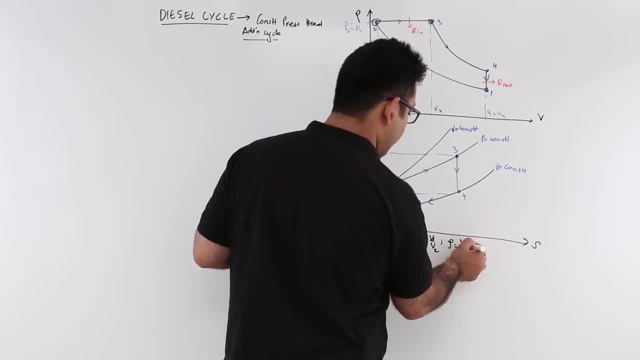 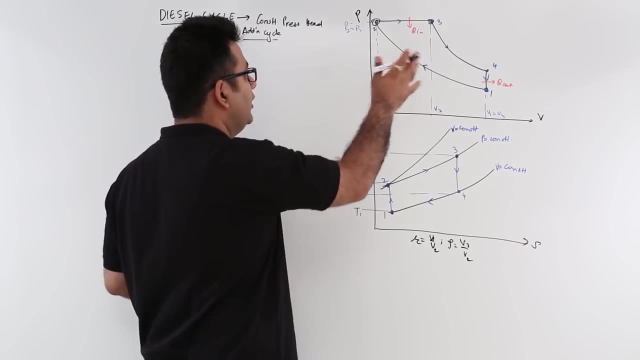 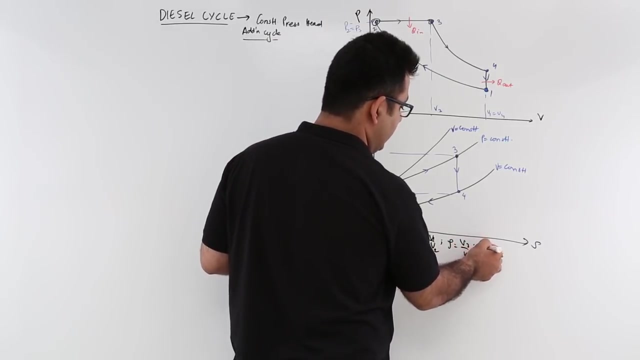 So the fuel starts to get supplied at 3.. So this becomes V3 by V2.. So you can see that there is some evident a volume increase during the fuel adhesion process. that is also known as the heat adhesion process. Next is expansion ratio RE. This is the expansion that takes place 3-4.. You'll have V4 by V3.. Ok, Now there is a. 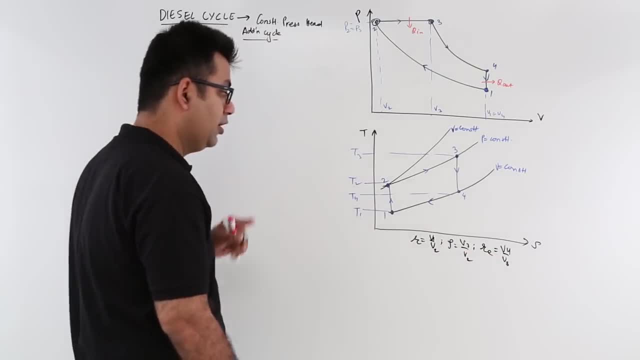 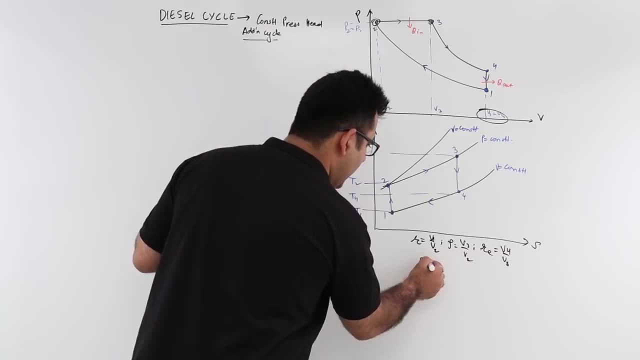 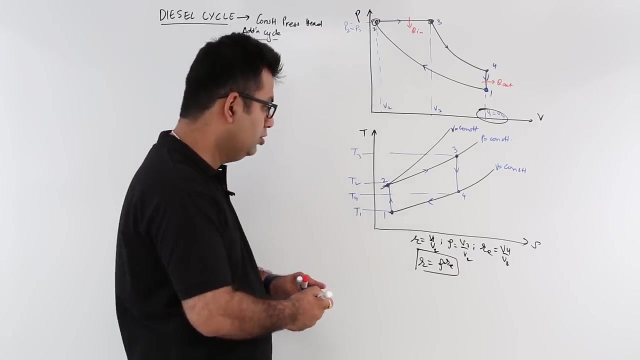 relation between these three ratios. that is also to be remembered. so we also know that V1 is equal to V4. so when you rearrange this, you will get R is equal to Rho into Re. so compression ratio is equal to fuel cut off ratio into the expansion ratio. okay, let's. 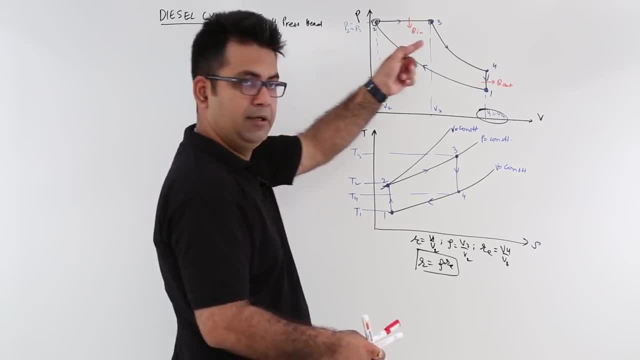 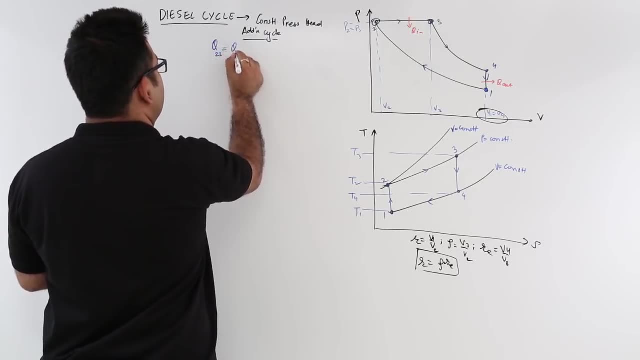 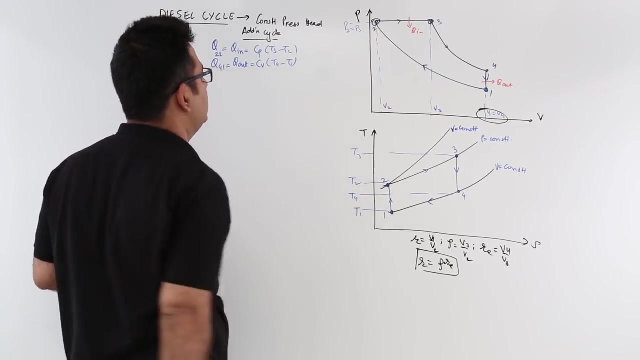 move forward with this. so let's look at the heat addition process, which takes place at constant pressure. so you have Q23, which is Qn, which is Cp, into T3 minus T2, and then you have Q41, which is Qout, which is Cv, into T4 minus T1. so this is what you have now when 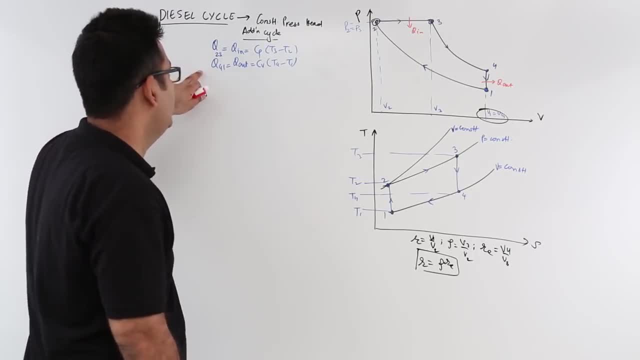 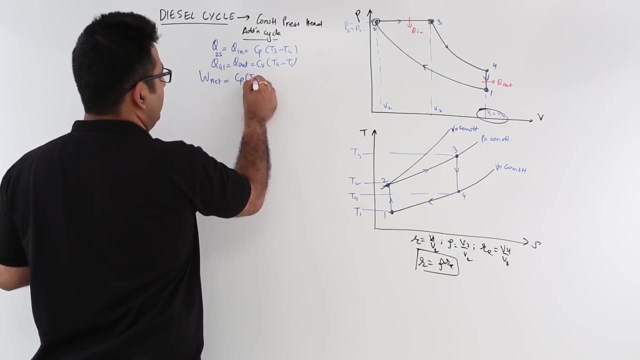 you find out the network, then that's a difference in these two heat values. so network output: this is Cp into T3 minus T2.. Minus Cv into T4 minus T1. if you divide this by Qn, so you have Cp into T3 minus T2. so this: 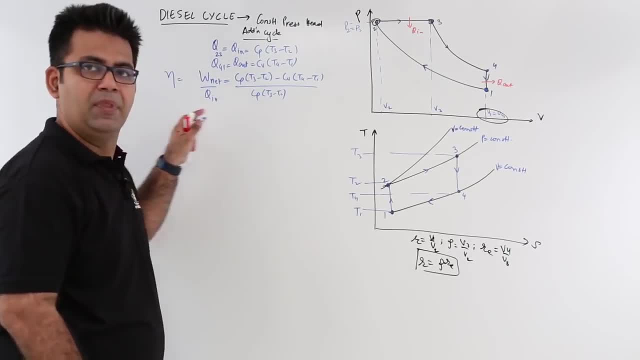 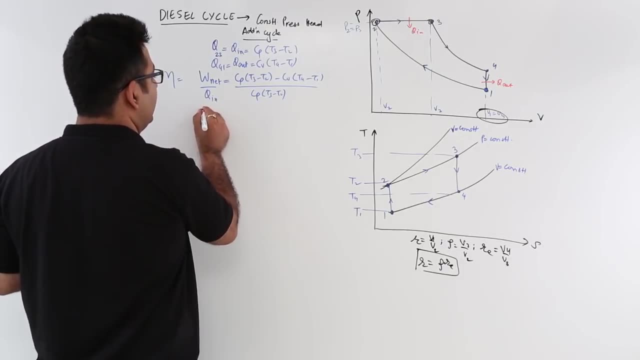 will give you the value of the efficiency of the diesel cycle. So this reduces this equation to something like this: so you have Cv upon Cp into T4 minus T1.. Minus Cp into T3 minus T2, divided by T3 minus T2.. 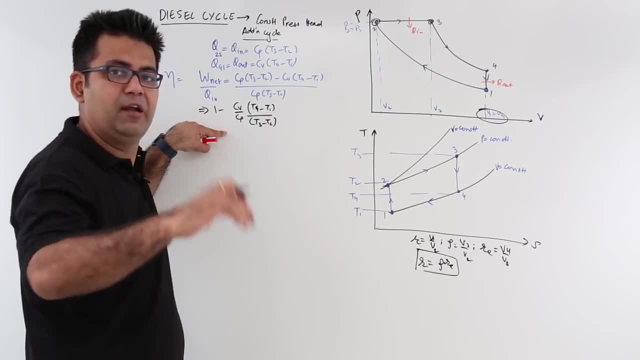 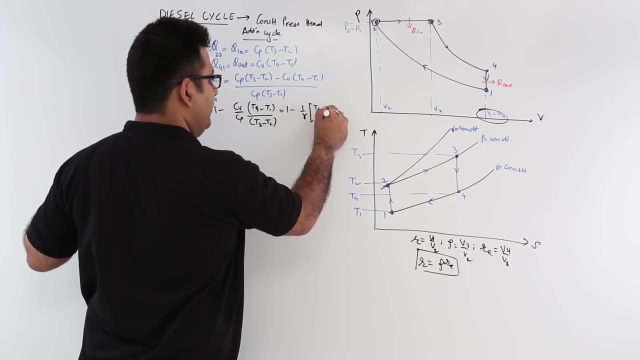 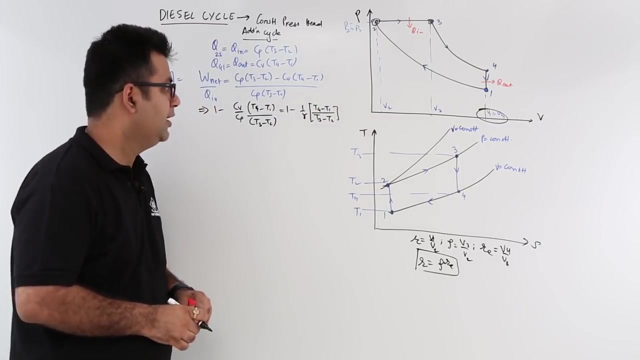 Now what is Cv upon Cp? that's the reciprocal of the adiabatic index. so that becomes 1 minus 1 by gamma, into T4 minus T1, divided by T3 minus T2. okay, Now again the question arises to get something out of them. okay, now how do we get that so? 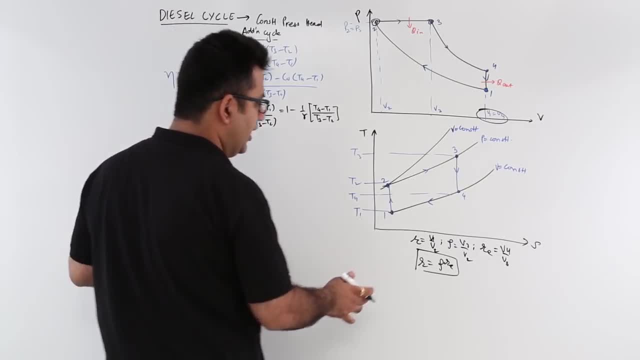 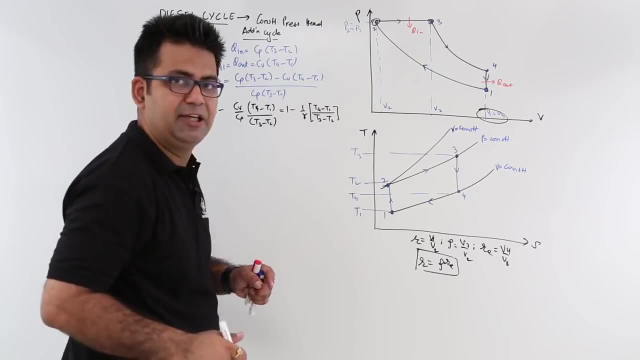 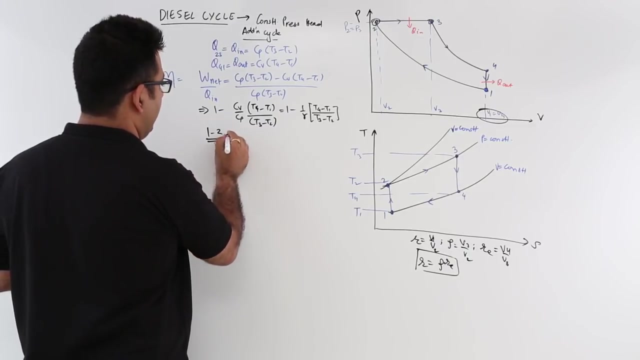 let's start. So we know that R is this, Rho is this and Re is that. okay, let's find out the analysis for the isentropic process: 1- 2. okay, So for 1- 2, if you apply the isentropic relation, so that is T2 by T1, which is equal to V1 by 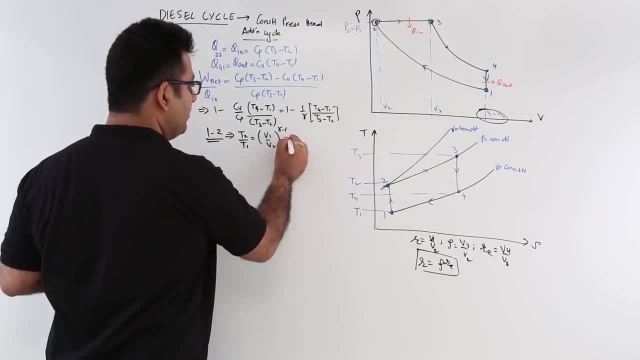 V to the power gamma minus 1. now, this is nothing but R to the power gamma minus 1, so this will give you the value of T2 in terms of T1 and R. okay, So this is an equation that we would like to use. 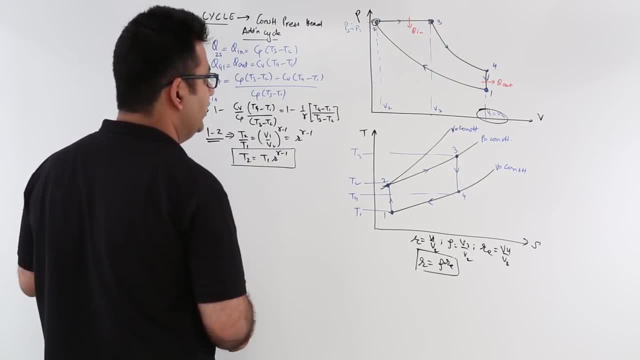 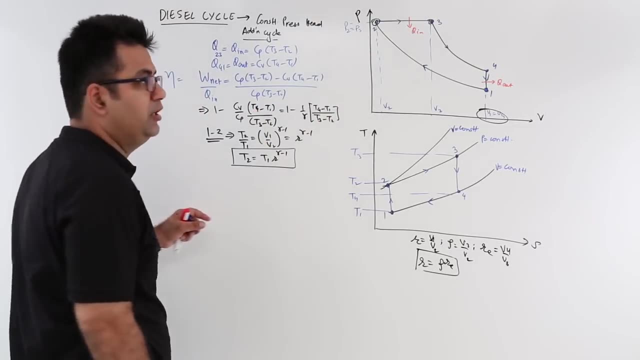 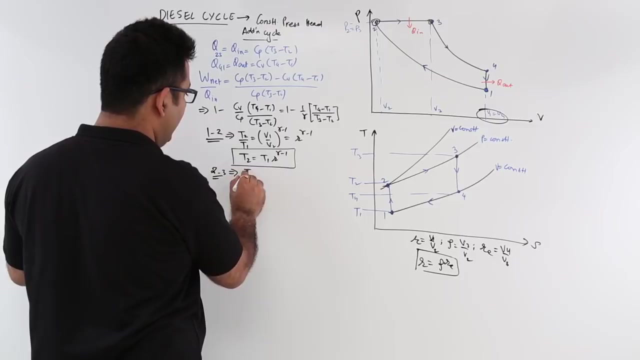 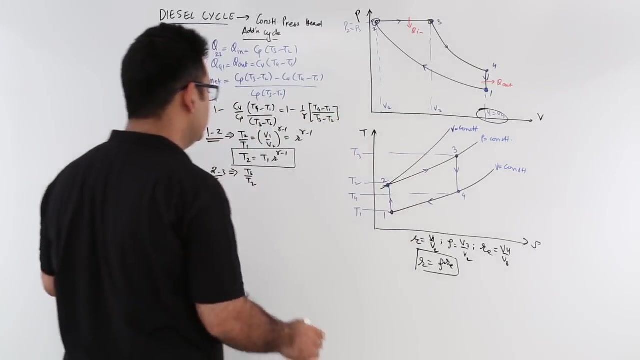 So let's put this into a box. Now let's use the fuel cutoff ratio, that is Rho. so if you take that isobaric process, 2, 3. So you will have T3. Okay, Okay Now, because the pressure is same, so I will need the volume ratios. So this is V3 by V2.. Now, V3 by V2, this is equal to rho. Now let's get the value for T3 now. 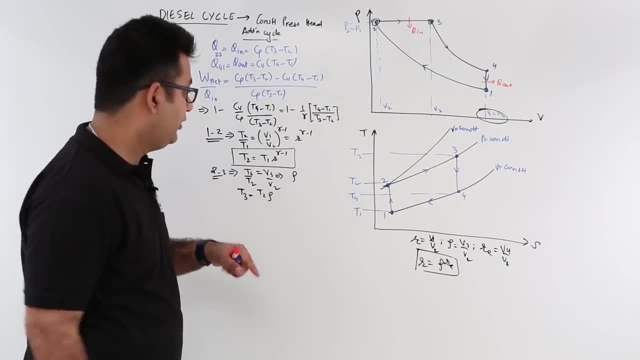 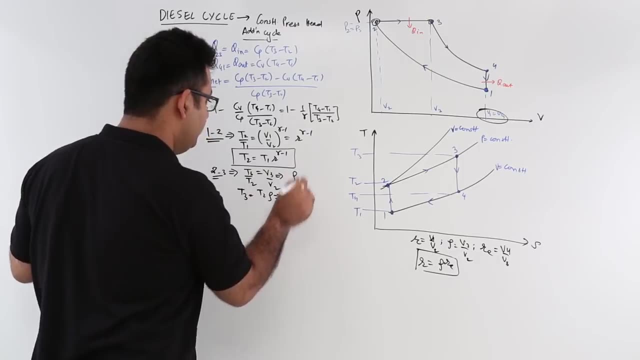 So T3 becomes T2 into rho. Now T2 already has a value in terms of T1 and R, So let's substitute that. So this gives you T3 is equal to T1 into R, to the power gamma minus 1 into rho. 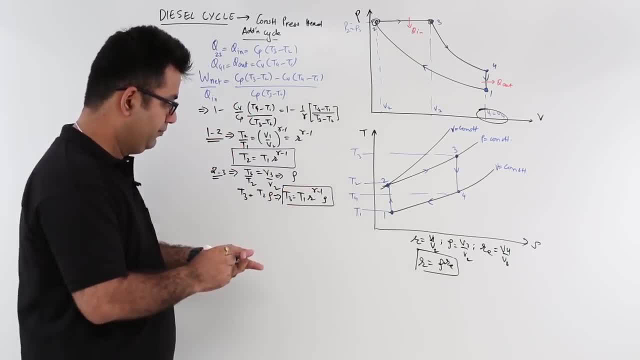 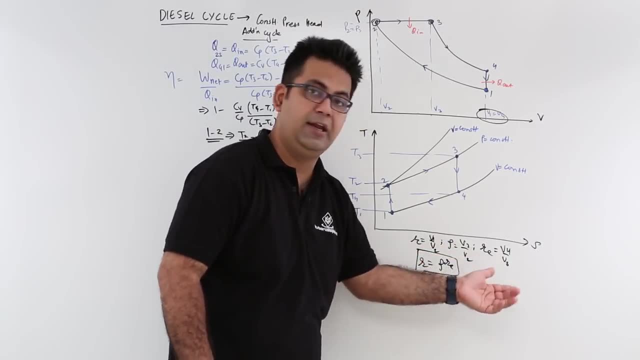 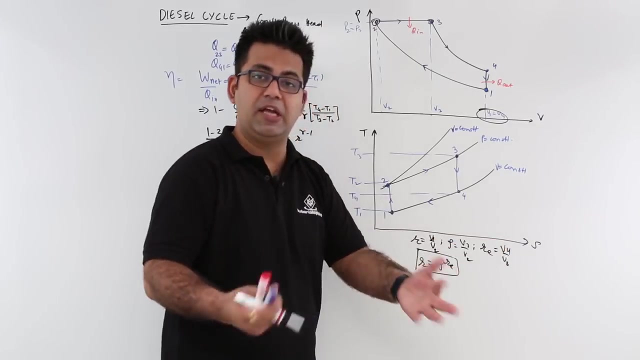 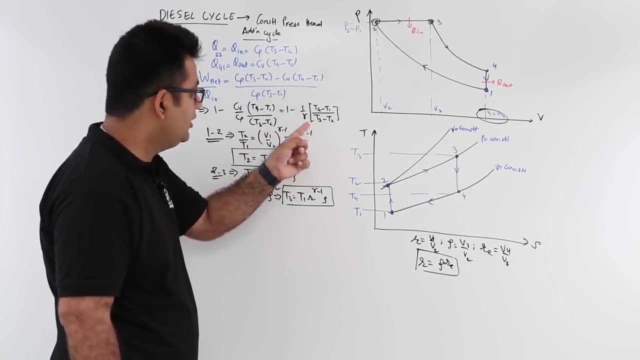 So that is another term we would be using for T3.. So now you see that these are, you know, constant values- R, rho and Re- for a given cycle, Right, Right? So as you change the Volumes and all these things, R, rho and Re would change If you change the operating conditions. Okay, So this means I am getting all these values, all these temperature values, in terms of one temperature. 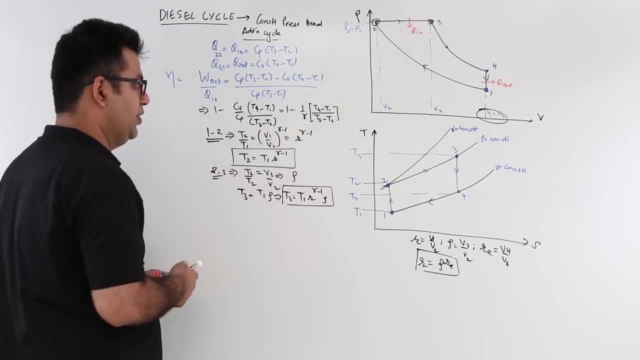 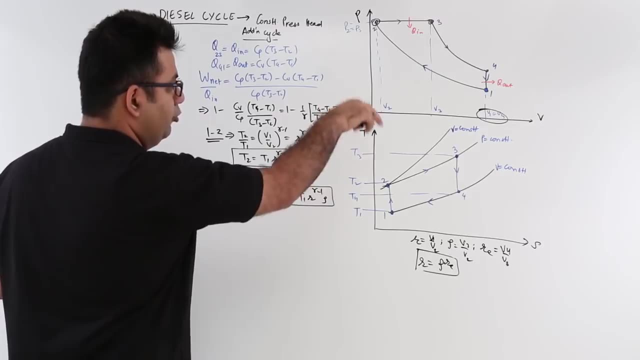 So I can cancel off that temperature from the entire equation. So I am done with T3 and T2 in terms of T1.. Now let's go to the process. 4, 1, or I would say 3, 4.. That's the isentropic expansion. 3, 4. first of all, 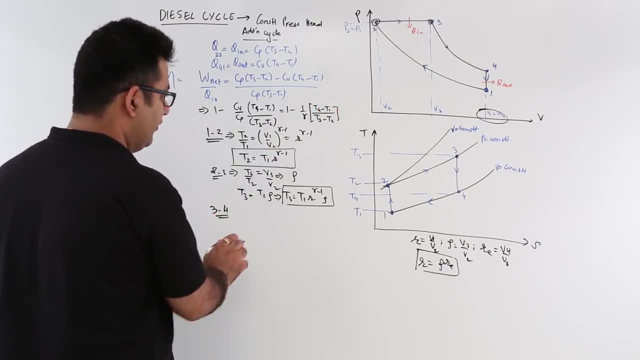 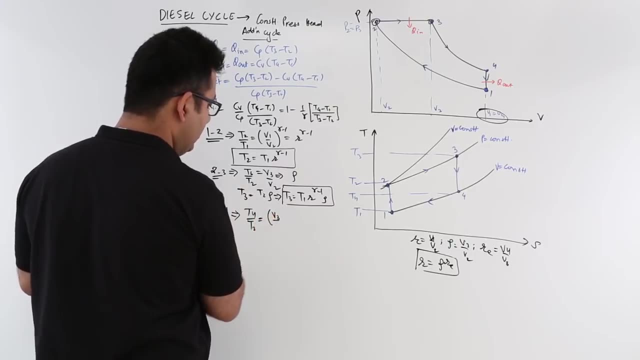 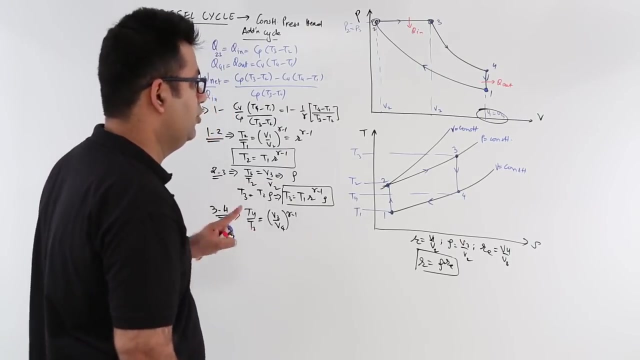 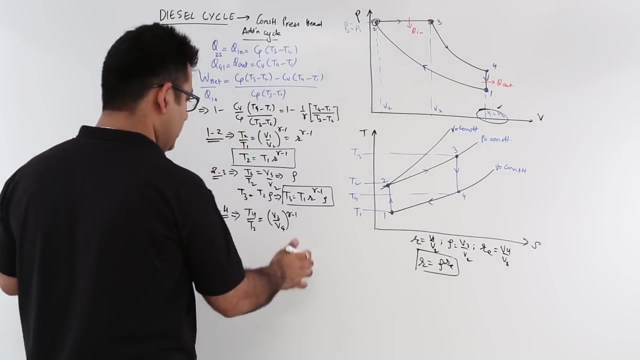 3, 4.. So this would give you T4 by T3. This is equal to V3 by V4 to the power gamma minus 1.. Now V3 by V4. Now, what is that? V3 by V4.. I know that V4 is equal to V1. So I can rewrite it as V3 by V1. 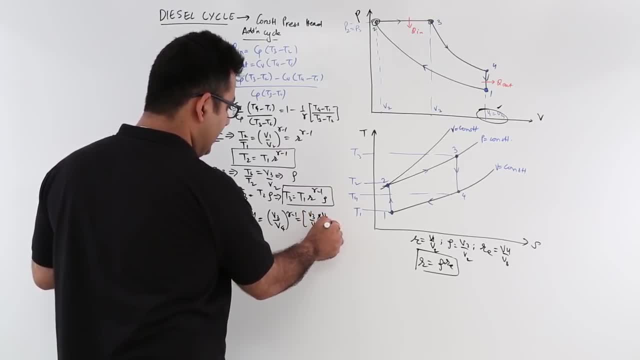 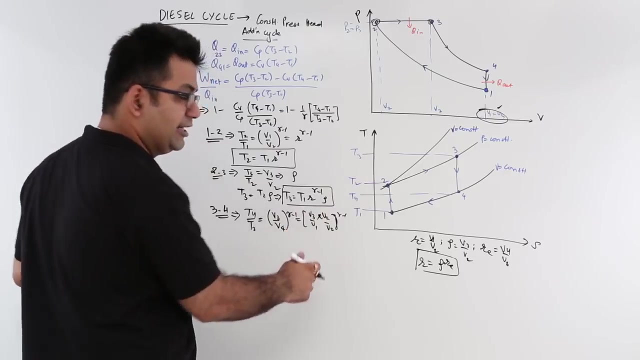 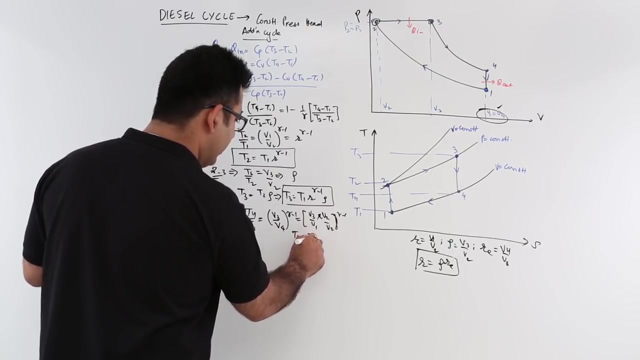 Okay, Okay, If I multiply and divide the entire ratio by V2, I can get something out of it. So what is V3 by V2?? V3 by V2 is rho, Okay. And what is V1 by V2?? So now this is the reciprocal of the compression ratio. So you will get T4 is equal to T3 into V3 by V2 is rho, So this becomes rho into gamma minus 1.. 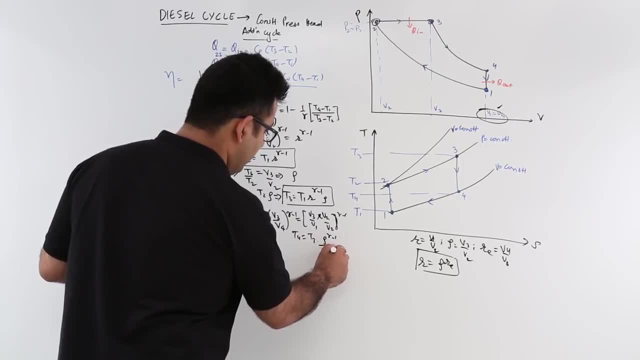 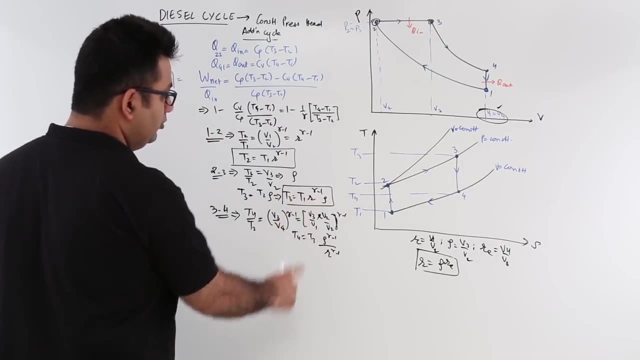 Upon R to the power gamma minus 1.. Because V2 by V1 is the reciprocal of R. Okay, Now, what is T3?? T3 is T1 into all these things. So let's get that value in terms of T1.. 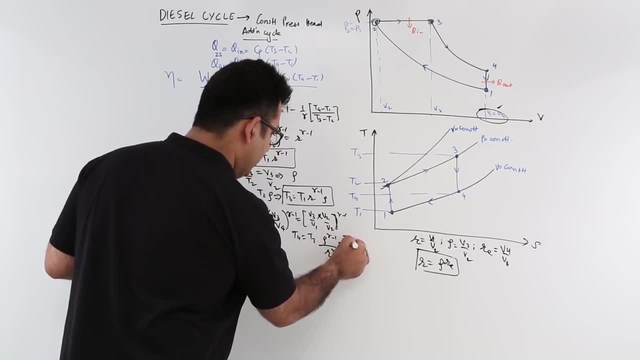 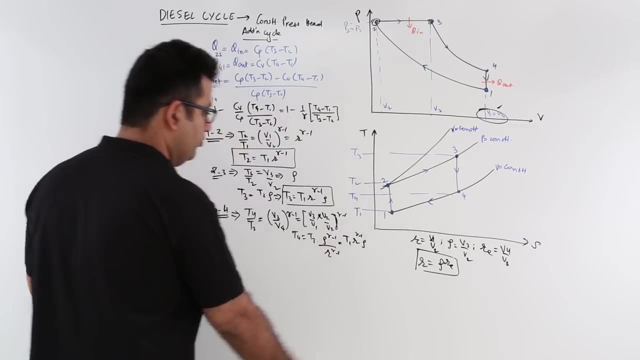 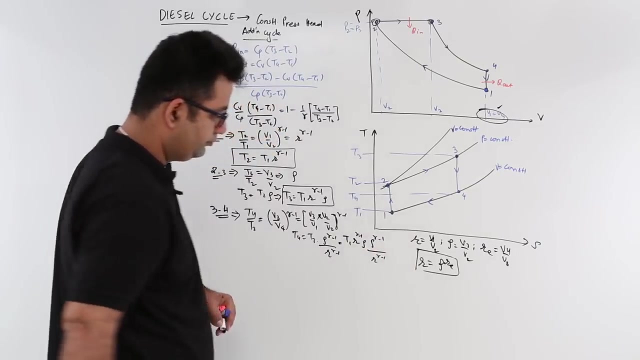 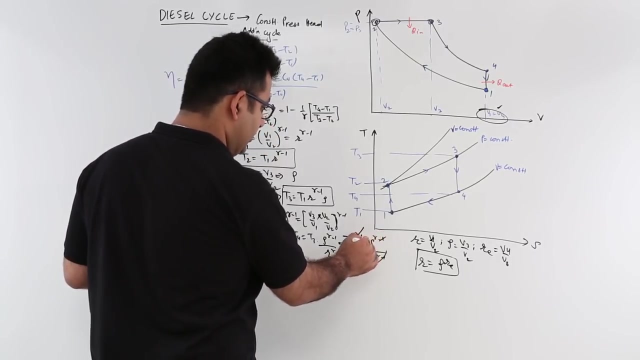 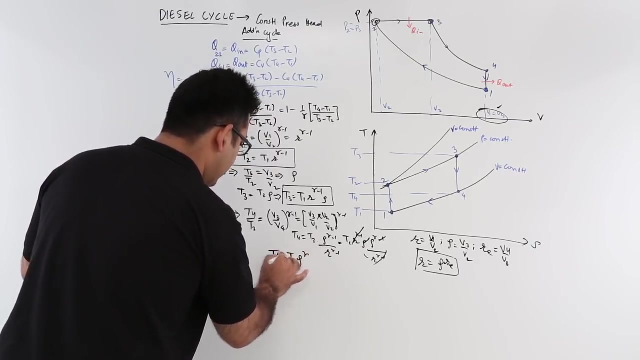 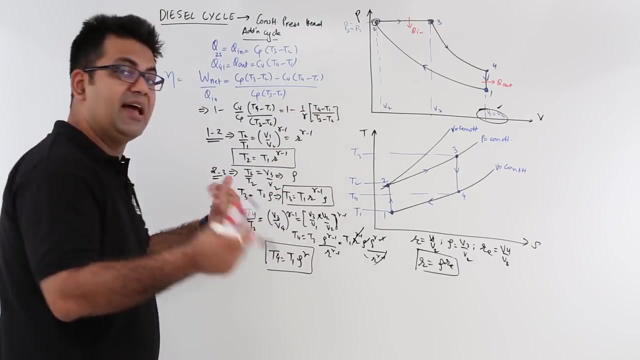 Okay, Gamma minus 1.. So this gets cancelled off, And then you can cancel off this and rho, So the value of T4 becomes T1, into rho to the power gamma. So now I have, you know, I have- four temperatures And now I have the value of three temperatures in terms of the four temperature. 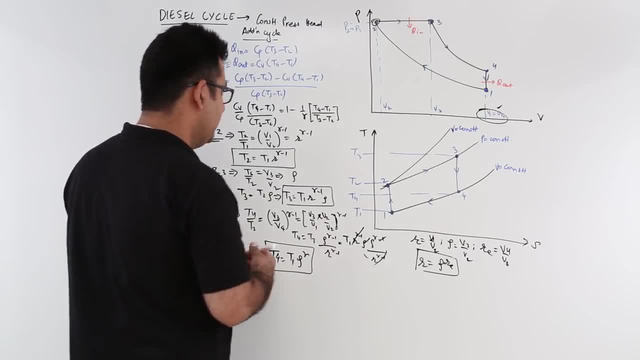 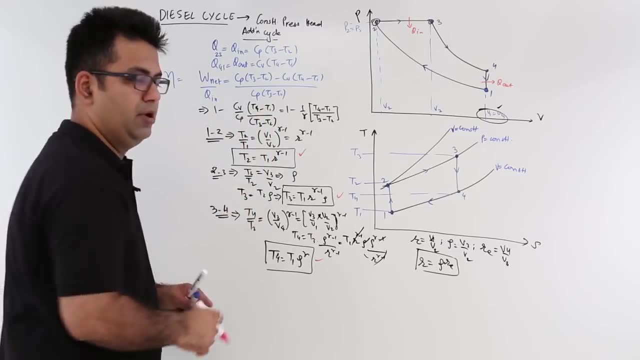 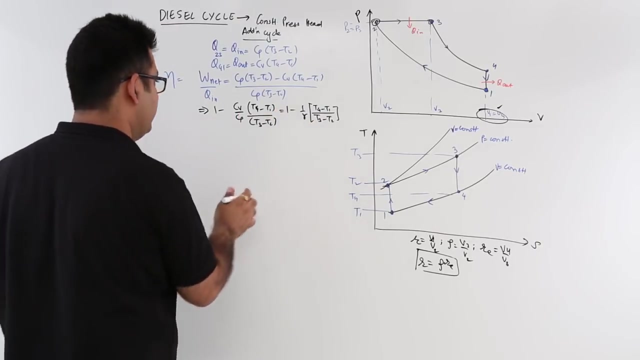 Okay, So I will be using This equation, this equation and this equation and put it into the you know expression for efficiency. Okay, So let's put the values of T4, T3 and T2 in this expression for efficiency, So you get 1 minus 1 by gamma. Okay, Into T4 is rho, to the power gamma, into T1. Okay. 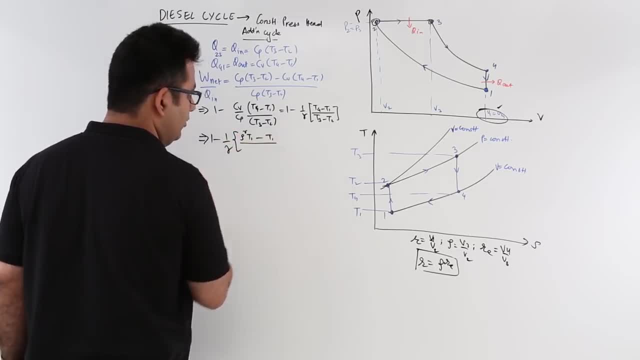 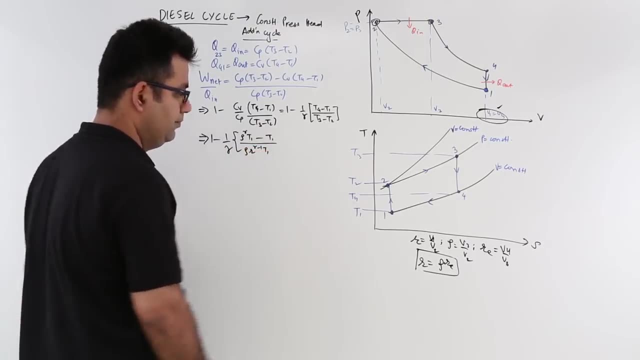 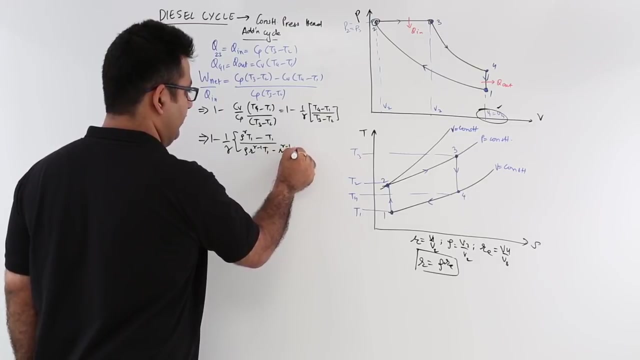 T1 will come as it is Upon T3.. T3 is: T3 is rho into R to the power gamma minus 1 into T1. Okay, And then T2 is R to the power gamma minus 1 into T1. So this is the entire expression that you get now.